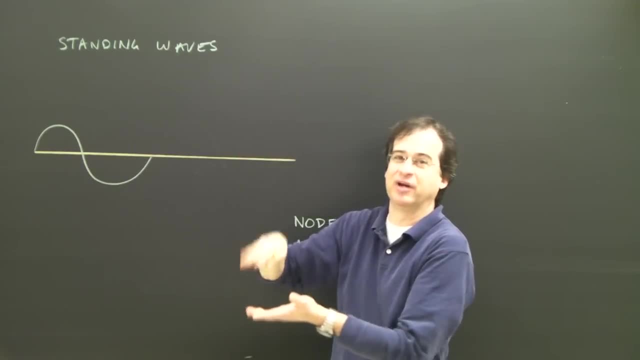 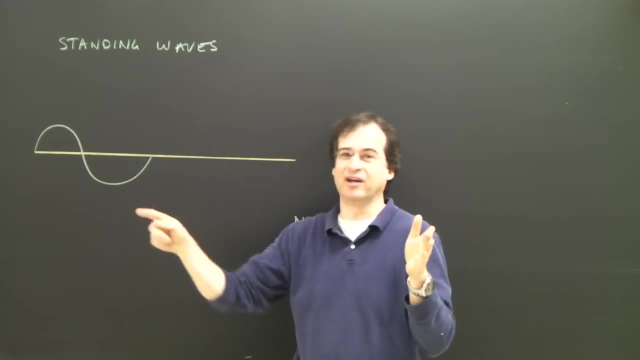 It doesn't look like the waves traveling back and forth. you just see it vibrating up and down. That's why we call it a standing wave. It's really created when a wave is traveling along a string, bounces off the other end and comes back. 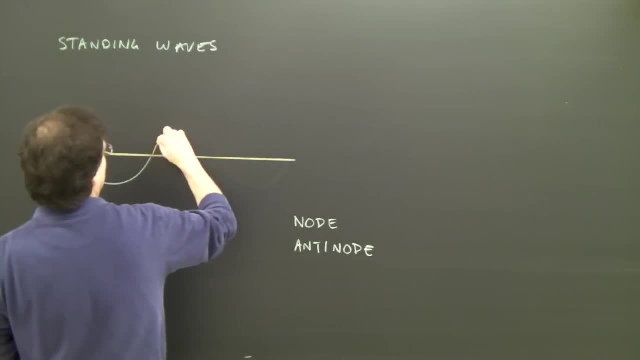 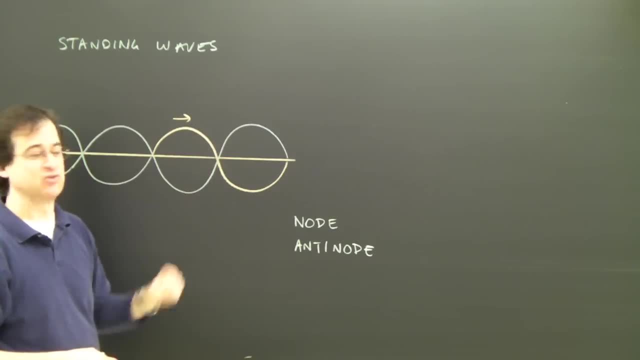 But at this point the guitar string will be sitting still, So it's called a standing wave. It's a spring or a string vibrating like this up and down. It's continually moving waves this way, but it just looks like the string is vibrating up and down. 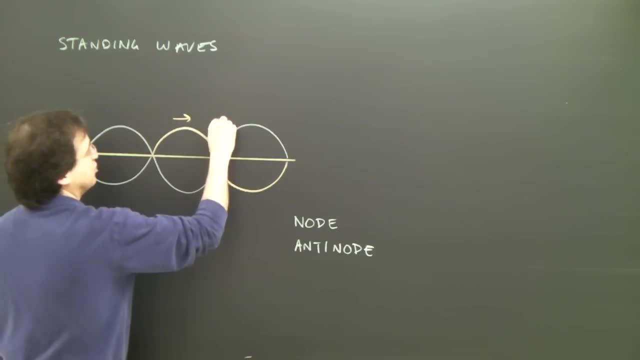 Now we have some parts. we need to label These. where the string is not moving, they're called nodes. The part where the string is moving up and down rapidly, that's called an antinode. So these are antinodes in that vibrating string. 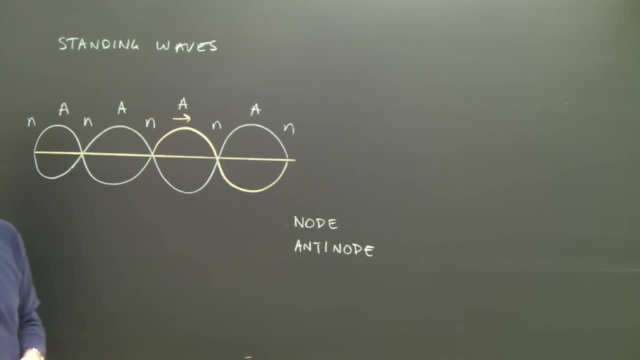 It doesn't always look like this. We don't necessarily always have four loops. Each one of these loops is made up of part of a wave. There's the wave that's creating it and since that's the wave that's creating it, that's the wavelength. 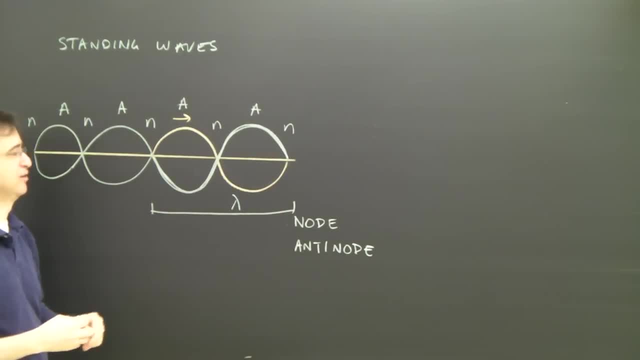 So two of these loops are equal to the wavelength, which means every node-to-node distance is half a wavelength. So if we have a guitar string and it's vibrating like this, simply vibrating up and down, we know that this is one-half lambda. 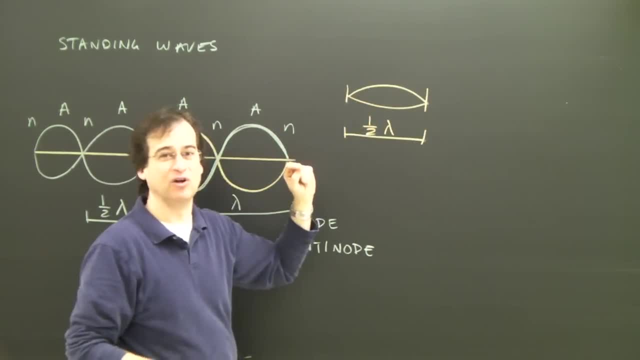 So if the guitar string is 30 centimeters long and you pluck it, how long is the wave that's making that sound? Well, if it's 30 centimeters from here to here, the node distance, that's half a wavelength. 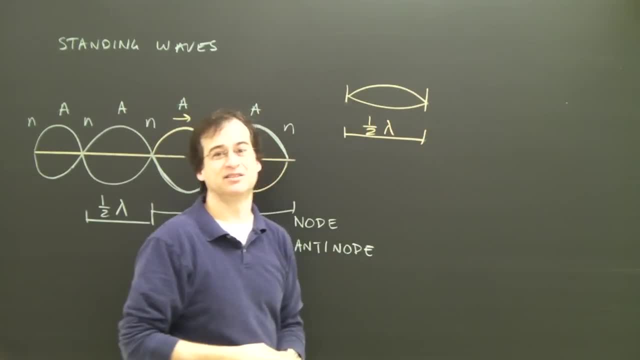 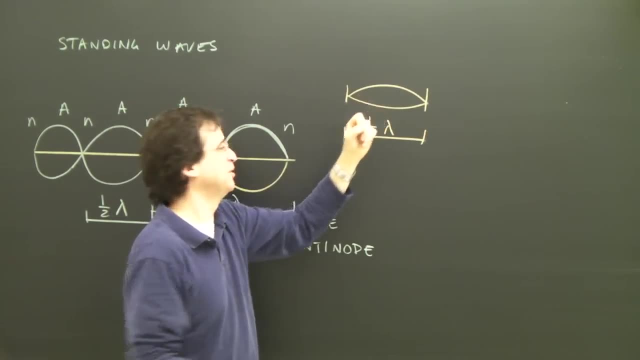 So then the wave must actually be double that 60 centimeters. So when I pluck a guitar string a certain way and I get this pattern of the string vibrating up and down, if the guitar string is 30 centimeters long, I know the wave is 60 centimeters.